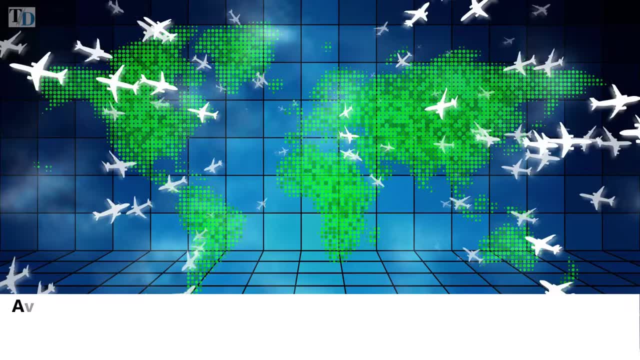 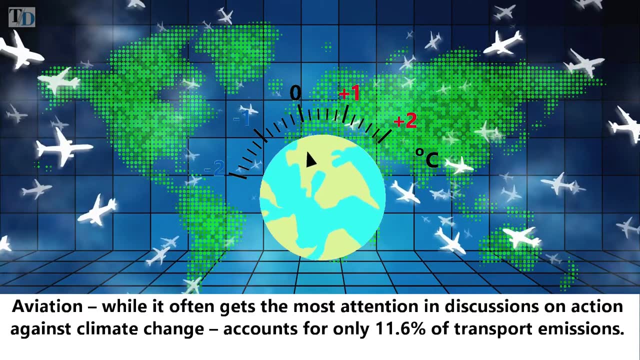 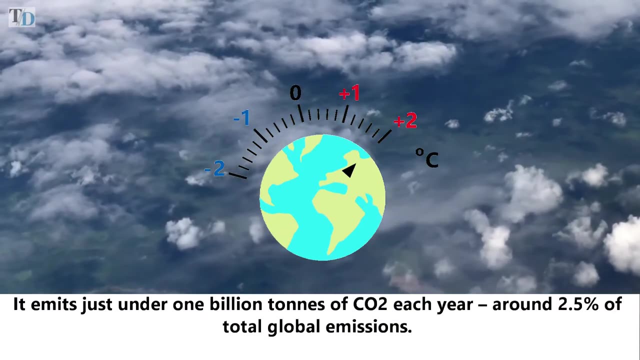 15 percent of total co2 emissions. aviation, while it often gets the most attention in discussions on action against climate change, accounts for only 11.6 percent of transport emissions. it emits just under 1 billion tons of co2 each year- around 2.5 percent of total global emissions. 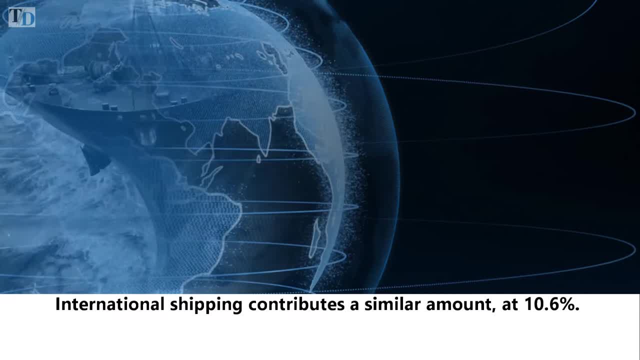 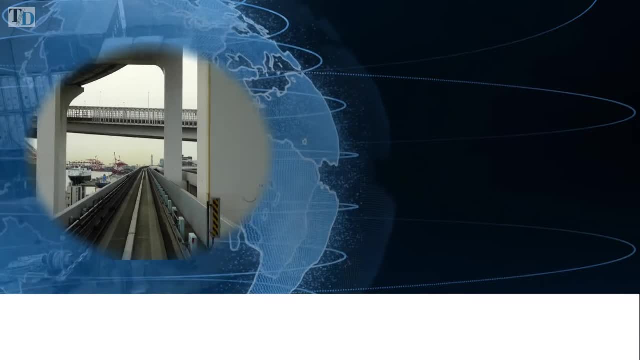 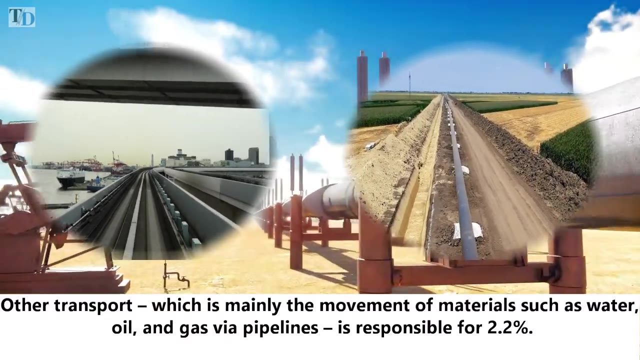 international shipping contributes a similar amount at 10.6 percent. rail travel and freight emit very little, only one percent of transport emissions. other transport, which is mainly the movement of materials such as water, oil and gas via pipelines, is responsible for 2.2 percent. transport demand is expected to grow across the world. 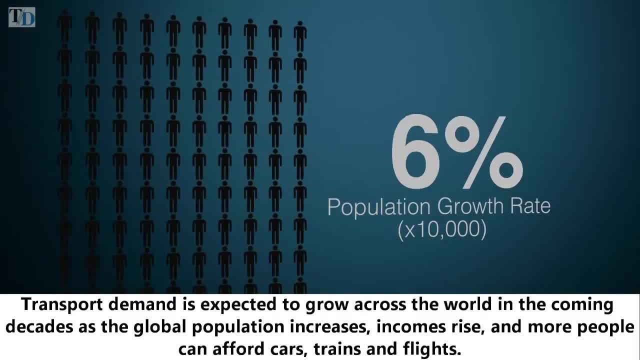 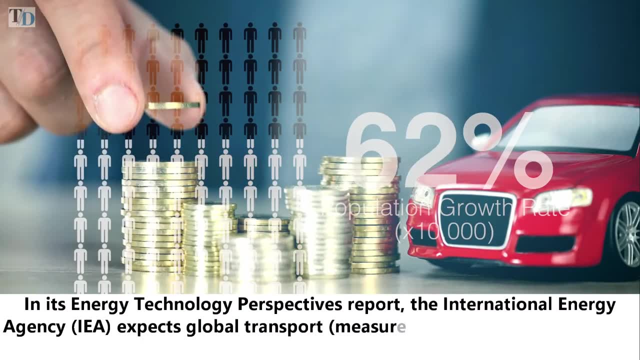 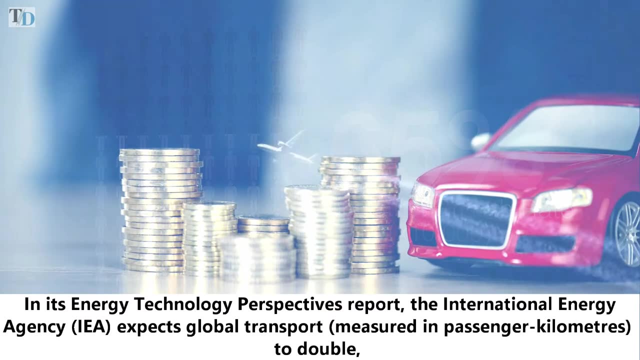 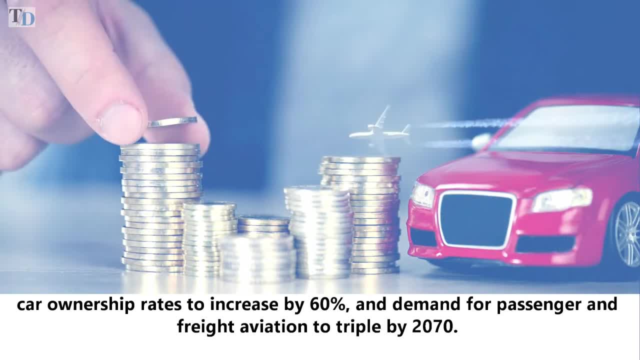 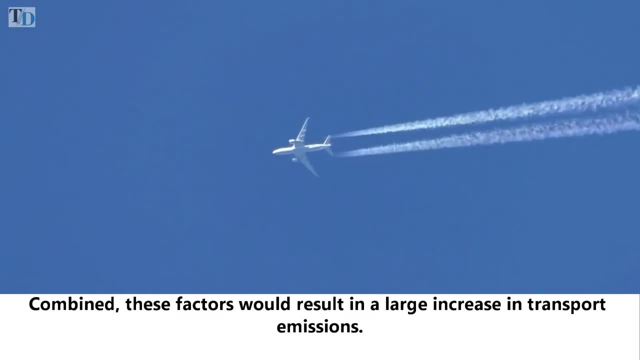 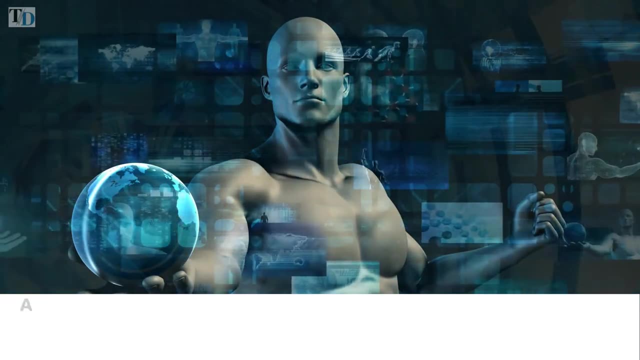 rates to increase by 60 percent and demand for passenger and freight aviation to triple by 2070. combined, these factors would result in a large increase in transport emissions, but major technological innovations can help offset this rise in demand as the world shifts towards lower carbon electricity sources. the rise of electric 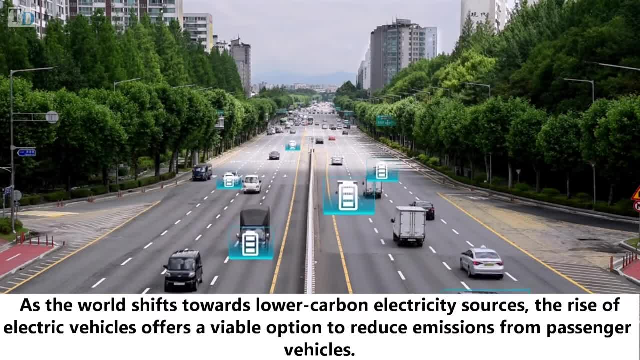 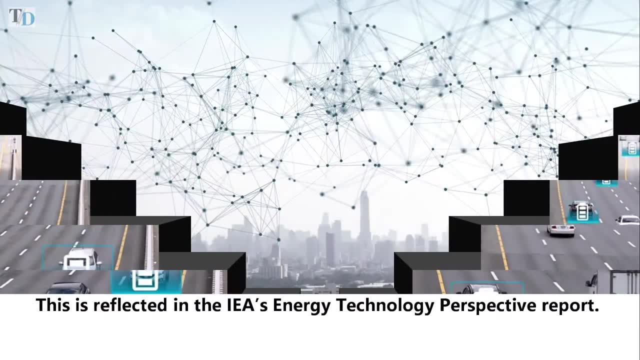 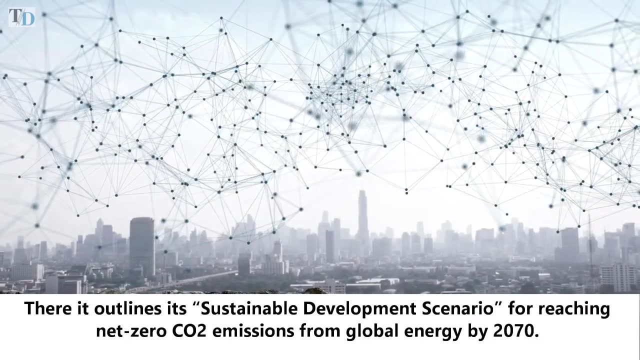 vehicles offers a viable option to reduce emissions from passenger vehicles. this is reflected in the iea's energy technology perspective report. there it outlines its sustainable development scenario for reaching net zero co2 emissions from global energy by 2070.. the pathways for the different elements of the transport sector. 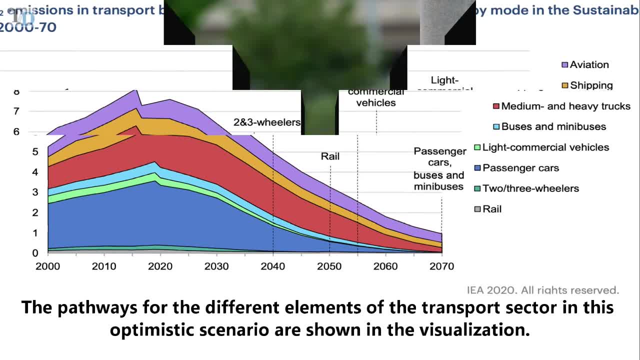 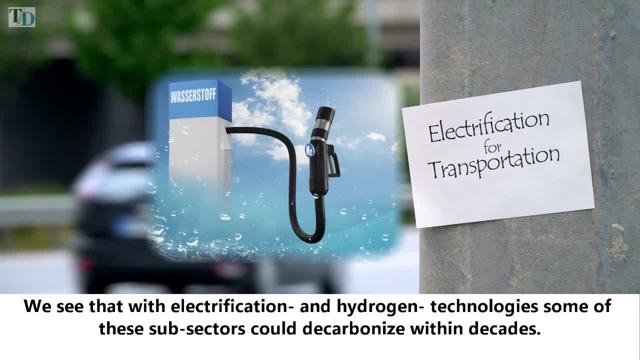 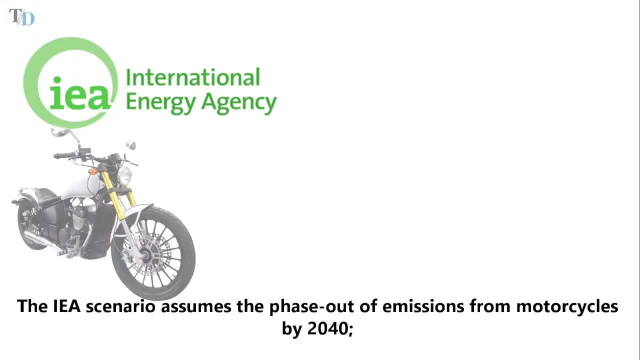 in this optimistic scenario are shown in the video. We see that with electrification and hydrogen technologies, some of these sub-sectors could decarbonize within decades. The IEA scenario assumes the phase out of emissions from motorcycles by 2040, rail by 2050, small trucks by 2060,. and although emissions from cars and buses are not completely eliminated until 2070,, it expects many regions, including the European Union, United States, China and Japan, to have phased out conventional vehicles as early as 2040.. Other transport sectors will be much more difficult to decarbonize.